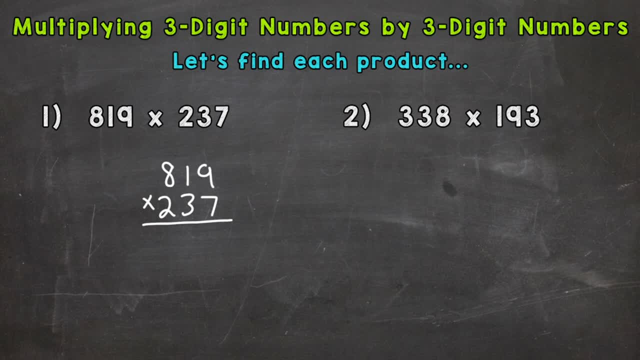 30 times 819, and then 200 times 819. add up to 819.. Add all of those up and that will give us our final answer. And I said 30 because that 3 in 237 is in the tens place. 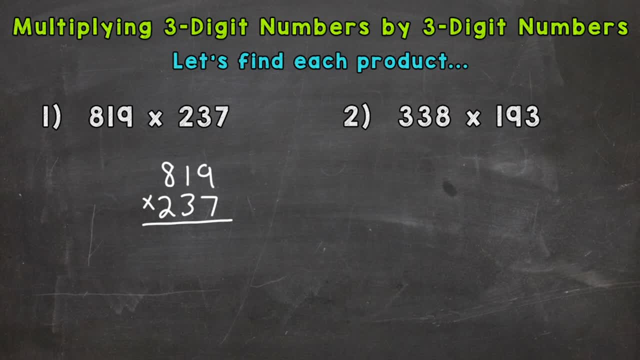 So it has a value of 30.. And I said 200 because that 2 in 237 has a value of 200, because it's in the hundreds place. So let's start, And we start by doing 7 times 9, which is 63.. 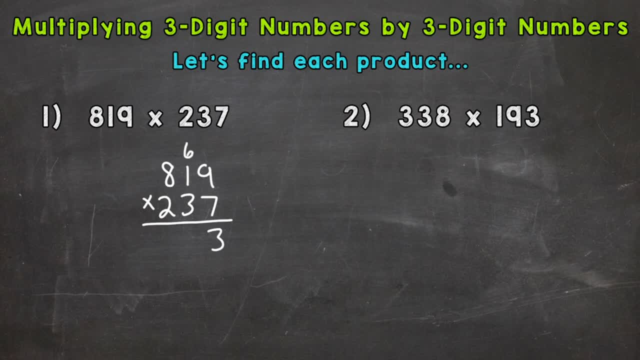 So we put our 3 and carry the 6.. Now we have 7 times 10.. But we can just think of it as 7 times 1 and look at these as the basic digits. Now I said 10 because that 1 is in the tens place, so it has a value of 10.. 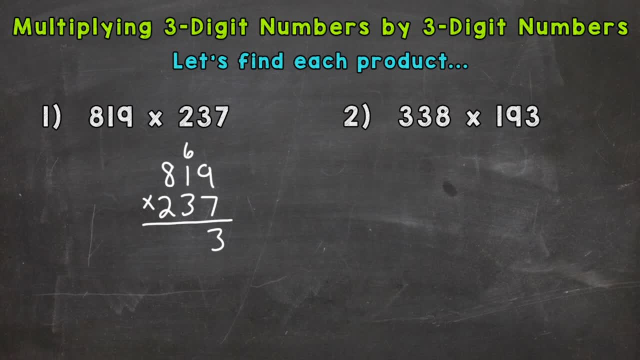 But let's just think of it as the digits themselves, like I said. So 7 times 1 is 7 plus 6 is 13.. So we put our 3 and carry the 1.. Now we have 7 times 800, but we can just think of it as 7 times 8, which is 56, plus that 1. 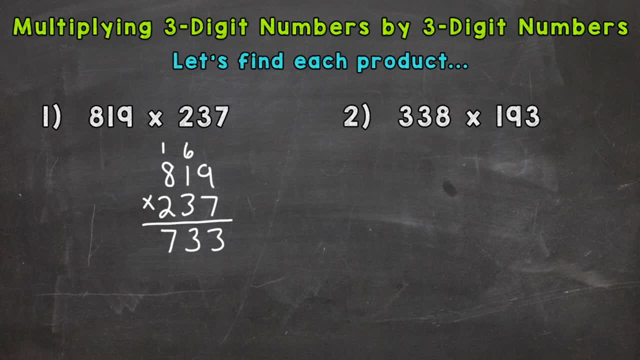 is 6.. So we put our 7 and we don't have any more digits to carry over to, So we drop our 5 and we get an answer of 5,733.. We are done with the 7 here, the 6, and the 1.. 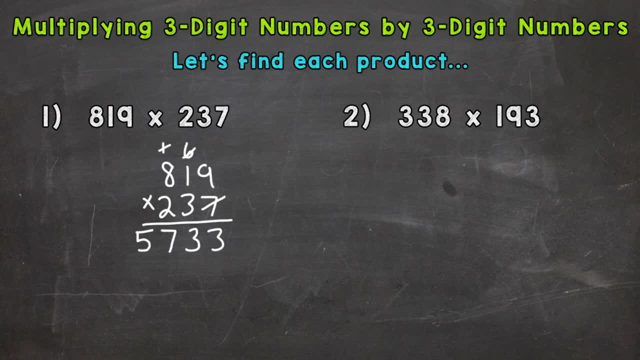 I like to cross things off as we go when we are done with them. That way we don't get confused with any other numbers that are carried later in the problem. So now we move to the 30 that has a value of. I'm sorry. we move to the 3 that has a value of 30. 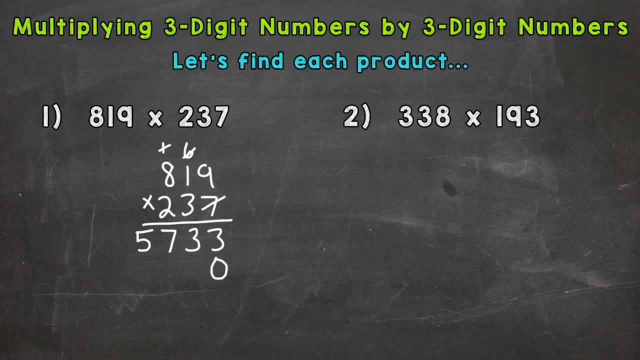 So we put a 0 here for our next step, and that represents that 30. It helps us represent the 30 rather than just saying it is a 3.. So now we do 3 times 9,, which is 27,. carry our 2.. 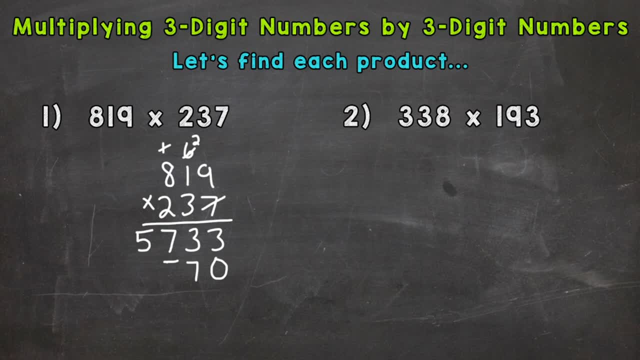 3 times 1 is 3, plus 2 is 5, and then 3 times 8 is 24.. So we are done. We are done with this 3 and then the 2.. So we move to the 2 in 237, which has a value of 200. 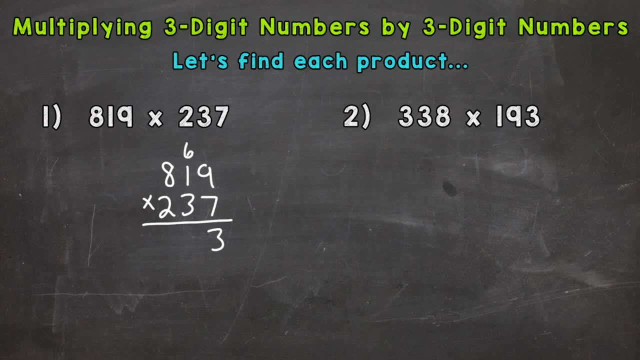 So we put our 3 and carry the 6. Now we have 7 times 10. But we can just think of it as 7 times 1 and look at these as the basic digits. Now I said 10 because that 1 is in the tens place. 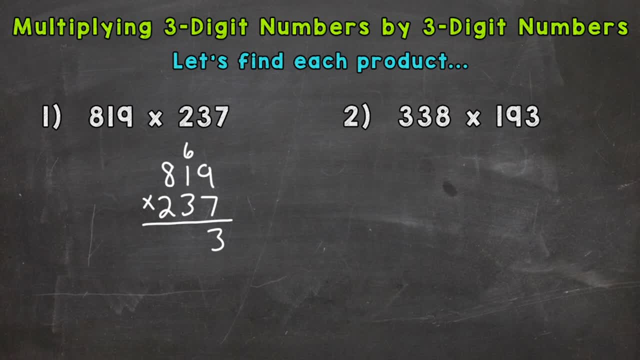 So it has a value of 10.. But let's just think of it as the digits themselves, like I said. So 7 times 1 is 7 plus 6 is 13.. So we put our 3 and carry the 1.. 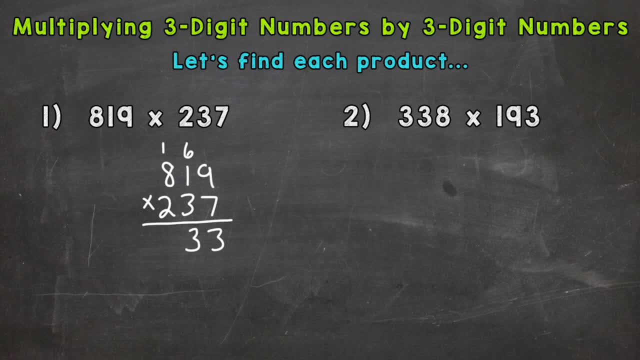 Now we have 7 times 800, but we can just think of it as 7 times 8,, which is 56, plus that 1. Is 57. So we put our 7 and we don't have any more digits to carry over to. 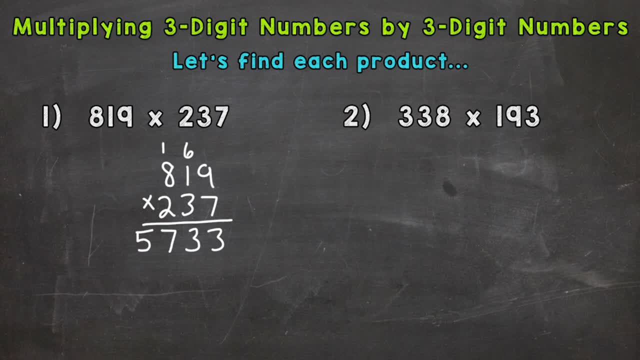 So we drop our 5 and we get an answer of 5,733.. We are done with the 7 here, the 6, and the 1.. I like to cross things off as we go when we are done with them. 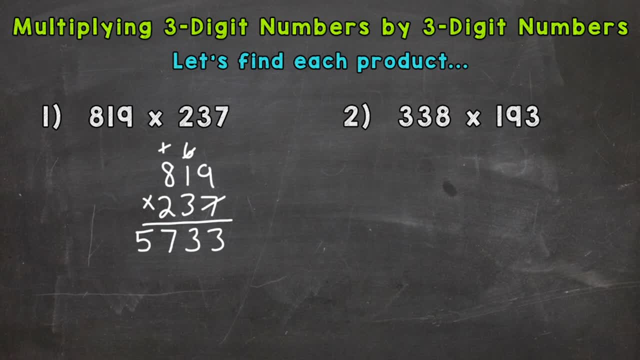 That way we don't get confused with any other numbers that are carried later in the problem. So now we move to the 30 that has a value of Or, I'm sorry, we move to the 3 that has a value of 30.. 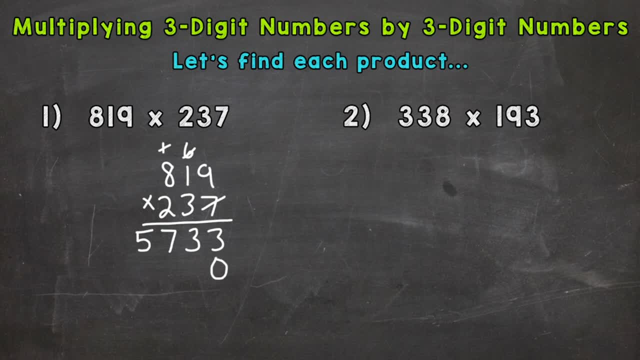 So we put a 0 here for our next step, And that represents that 30. It helps us represent the 30 rather than just saying it is a 3.. So now we do 3 times 9,, which is 27.. 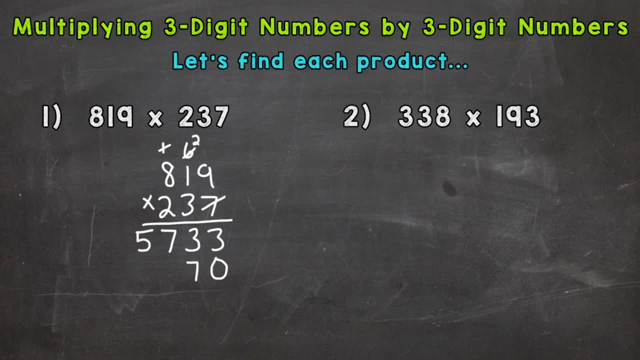 Carry our 2.. 3 times 1 is 3 plus 2 is 5.. And then 3 times 8 is 24.. So we have a 3.. We have a 7.. So we are done with this 3.. 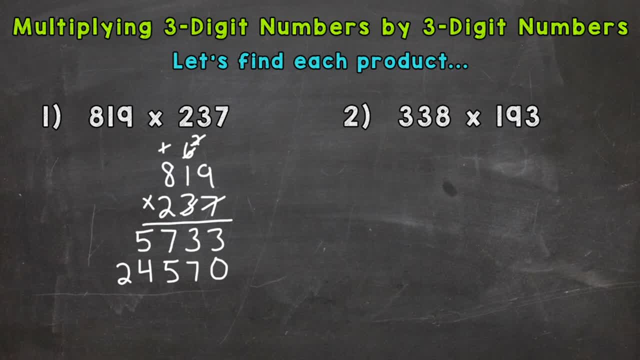 And then the 2.. So we move to the 2 in 237, which has a value of 200.. It's in the hundreds place, So we need two 0s for this next number Again, that's to represent the 200. 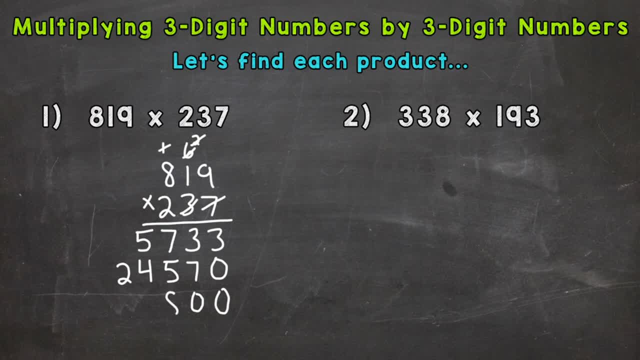 So now we do: 2 times 9 is 18.. Carry the 1. 2 times 1 is 2. plus that 1 is 3.. And then we have 2 times 8, which is 16.. So now we can add all of these up. 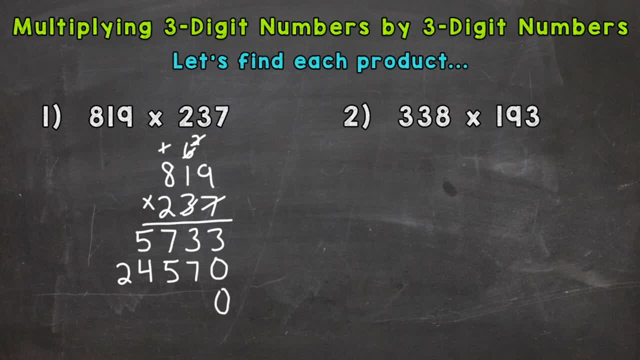 It's in the hundreds place. So we need two 0s for this next number. Again, that's to represent the 200.. So now we do: 2 times 9 is 18,, carry the 1.. 2 times 1 is 2,, plus that 1 is 3.. 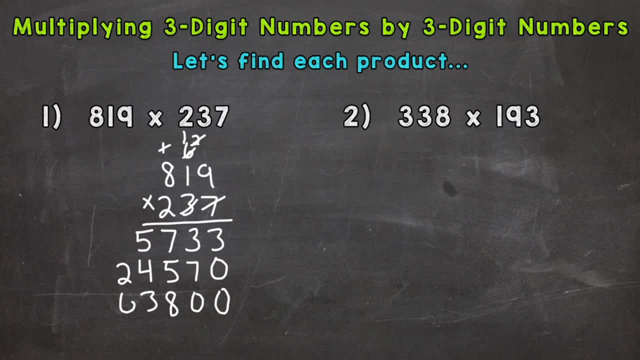 And then we have 2 times 8.. So now we can add all of these up. These are our partial products, So they are part of our final product or answer there. Add them up and we get our final answer. So 3 plus a couple of 0s, there is 3.. 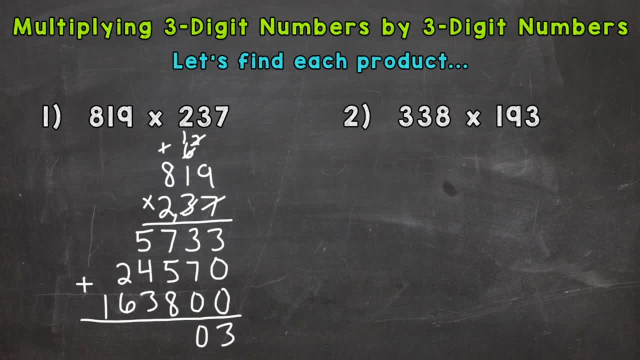 3 plus 7 is 10.. Carry our 1.. 1 plus 7 is 8, plus 5 is 13,. plus 8 is 21.. 2 plus 5 is 7, plus 4 is 11, plus 3 is 14.. 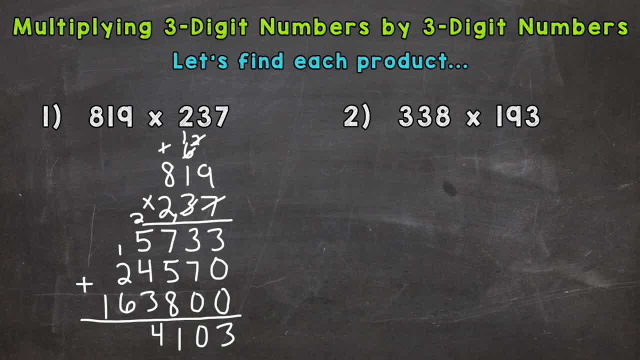 1 plus 2 is 3, plus 6 is 9.. And then we end with a 1 here And we get a final answer of 194,103.. So on to number 2, and we can line up our problem. 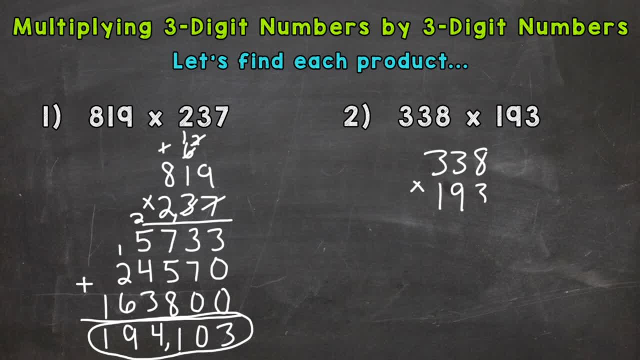 338 times 1 is 3.. 338 times 193.. So let's go through our steps and we will go a little quicker as we work through number 2.. 3 times 8 is 24.. 3 times 3 is 9, plus 2 is 11.. 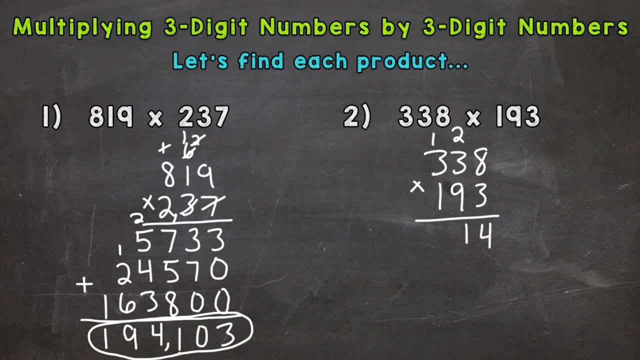 3 times 3 is 9, plus 1 is 10.. So we are done, done and done. We move to the 9,, which has a value of 90. So we need a 0 here. 9 times 8 is 72.. 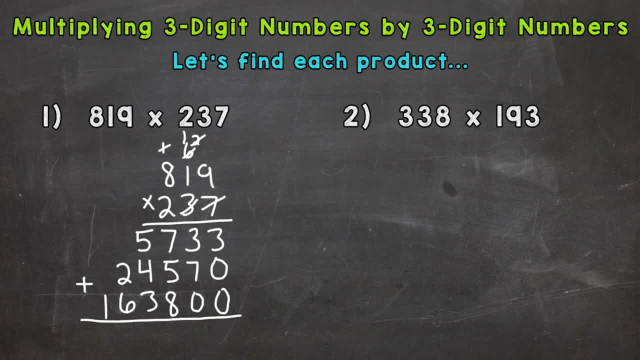 These are our partial products. So they are part of our final product or answer there. Add them up and we get our final answer. So 3 plus a couple of 0s, there is 3.. 3 plus 7 is 10.. 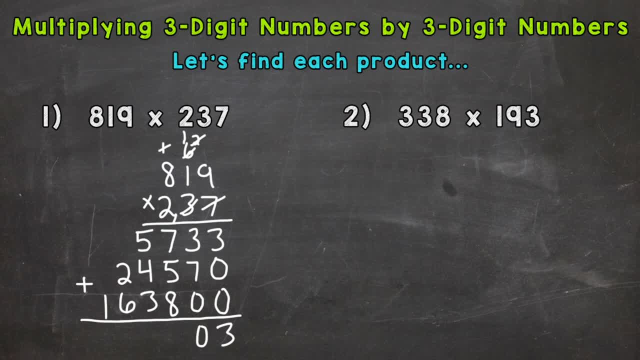 Carry our 1.. 1 plus 7 is 8.. Plus 5 is 13.. Plus 8 is 10.. Plus 8 is 21.. 2 plus 5 is 7.. Plus 4 is 11.. 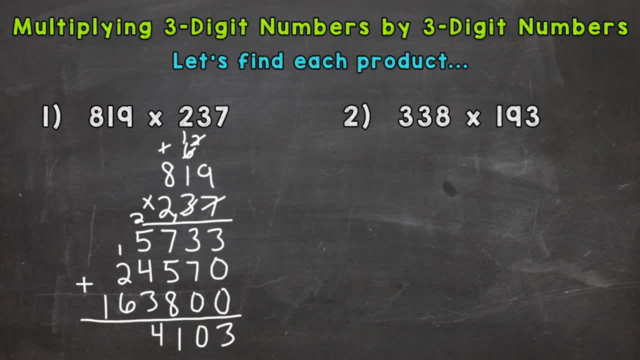 Plus 3 is 14.. 1 plus 2 is 3.. Plus 6 is 9.. And then we end with a 1 here And we get a final answer of 194,103.. So on to number 2.. 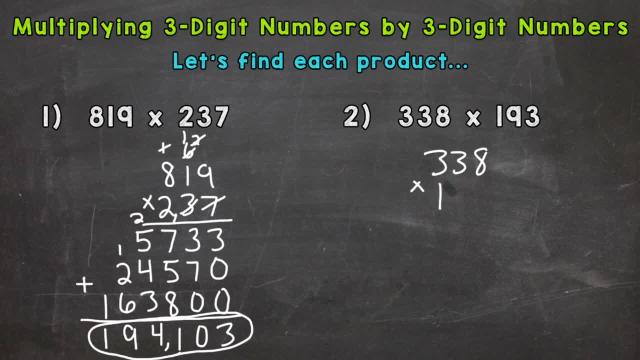 And we can line up our problem 338 times 193.. So let's go through our steps and we will go a little quicker as we work through number 2.. 3 times 8 is 24.. 3 times 3 is 9.. 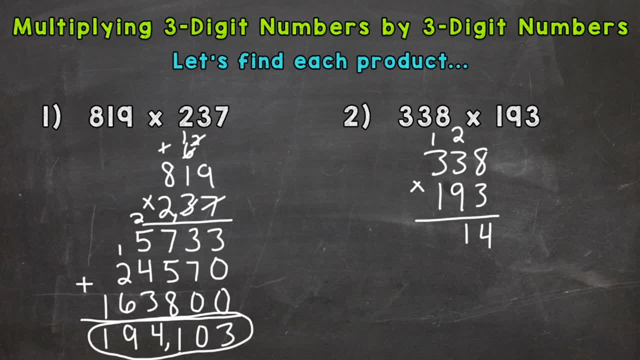 Plus 2 is 11.. 3 times 3 is 9.. Plus 1 is 10.. So we are done, done and done. We move to the 9,, which has a value of 90. So we need a 0 here. 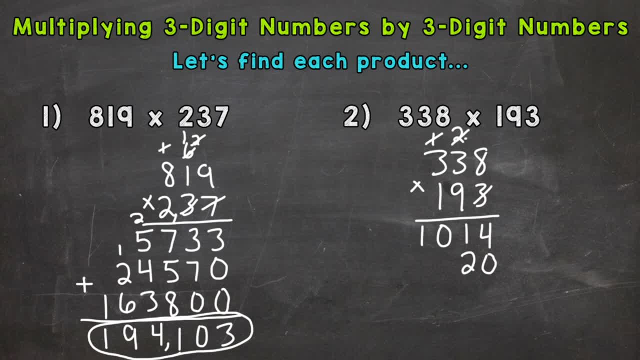 9 times 8 is 72.. 9 times 3 is 27.. Plus 7 is 34.. 9 times 3 is 27.. Plus 3 is 30. So we are done here, done here and done here. 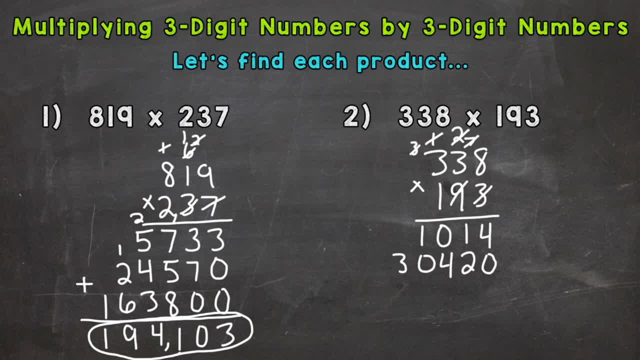 Now we have 100 times 338.. So that 1 has a value of 100.. So we need two 0s now. 1 times 8 is 8.. 1 times 3 is 3.. And 1 times 3 is 3.. 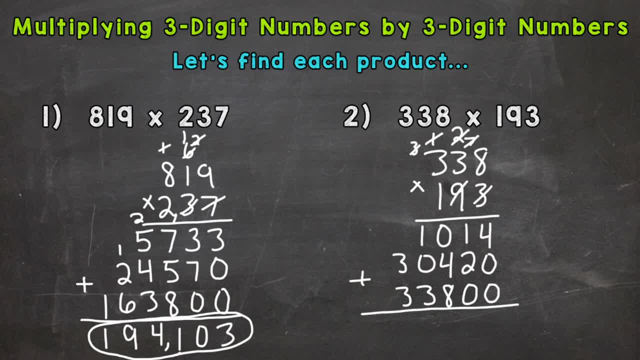 So we have our three partial products and we are ready to add them up in order to get our final answer. So 4 plus 0 plus 0 is 4.. 1 plus 2 plus 0 is 3.. 0 plus 4 is 4.. 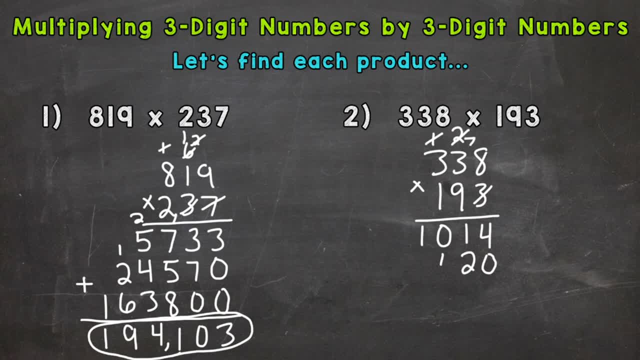 9 times 3 is 27,, plus 7 is 34.. 9 times 3 is 27,. plus 3 is 30.. So we are done here, done here and done here. Now we have 100 times 338.. 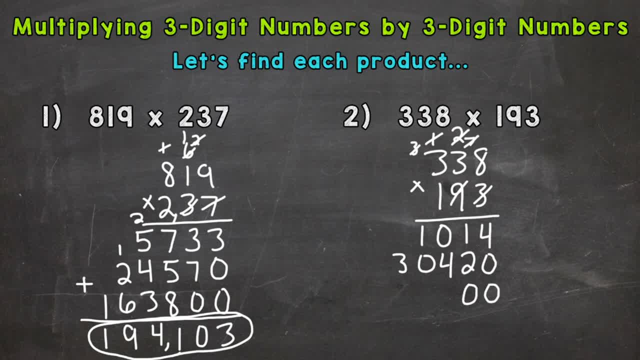 So that 1 has a value of 100, so we need two 0s now. 1 times 8 is 8.. 1 times 3 is 3, and 1 times 3 is 3.. So we have our three partial products and we are ready to add them up in order to get our final answer. 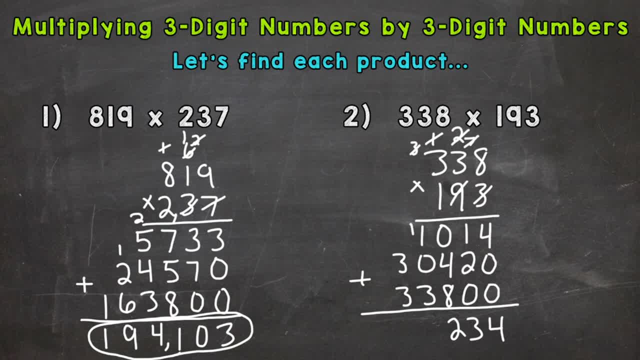 Plus 8 is 12.. 1 plus 1 is 2.. Plus 3 is 5.. And then we end with 3 plus 3. Which is 6.. So we get 65,234.. So there you have it. 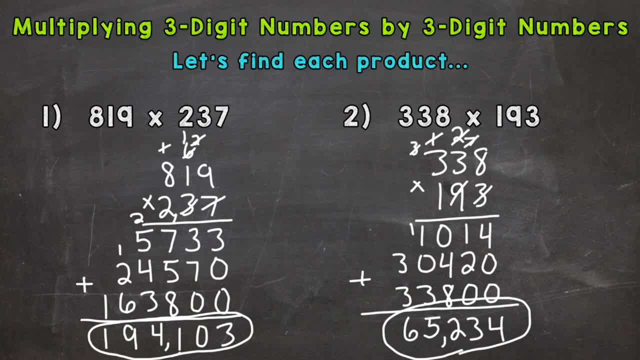 There's how you multiply three digit numbers by three digit numbers. I hope that helped. Thanks so much for watching. Until next time, peace. 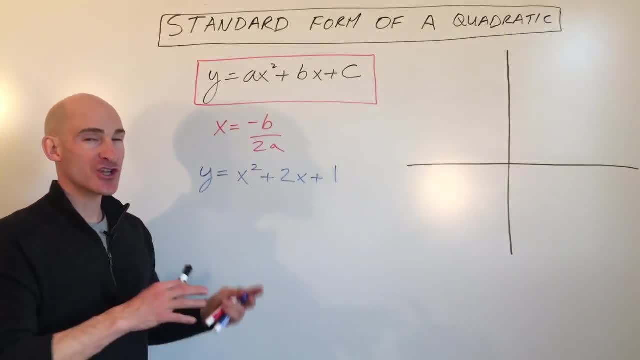 This is the standard form. Okay, now some books call it the general form and they call the standard form the vertex form. So you might want to take a look at your textbook and see if you need to refer to my video on the vertex form of a quadratic. But for purposes here we're just 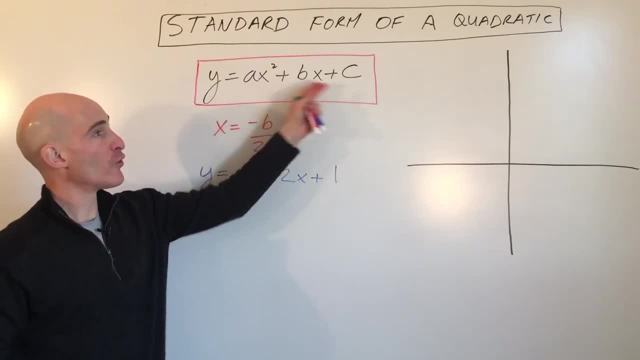 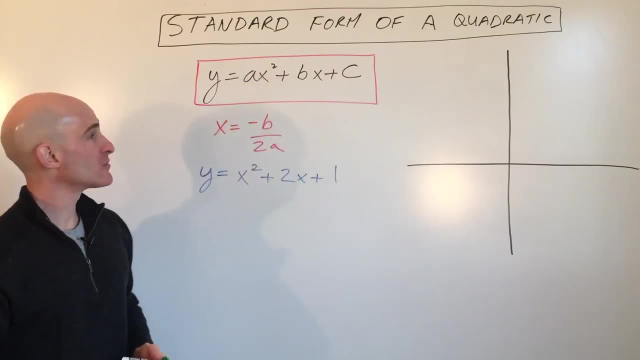 going to call this the standard form. This is just the foiled form or the descending form, where you can see it's going in descending order with the degrees of each term. But let's take a look at how to actually graph a parabola when it's in this, this form. Well, what you want. 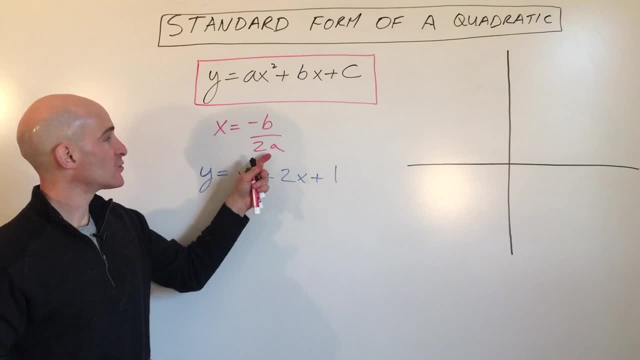 to do is: you want to find the vertex, and to find the vertex, we're going to start off by finding the x coordinate of the vertex, and the way we do that is by using this formula: x equals negative b over 2a. So you can see the coefficients. okay, those are your variables: a, b and c. So we're going to do. 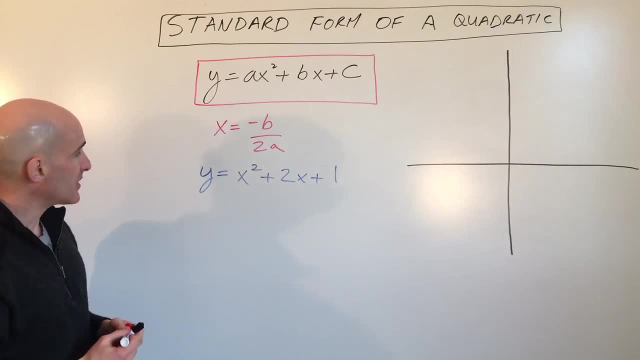 negative b over 2a to find our x coordinate of our vertex. So you can see, here this is going to be a and b and c. So we're going to do a and b and c, and we're going to do a and b and c. 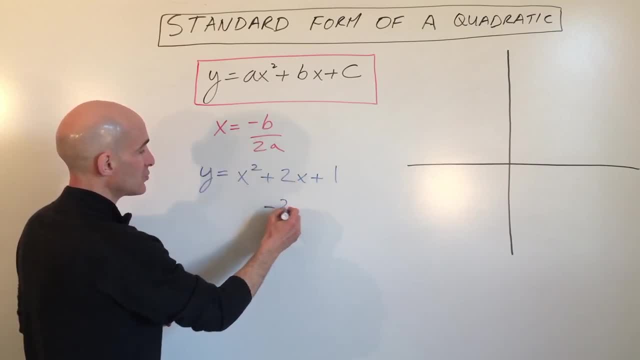 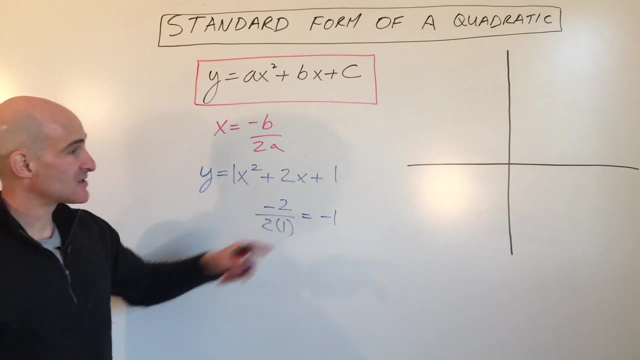 the b value. so negative two times, two times one. you see there's a one in front of the x squared, that's one. so that's going to come out to negative one. so what that means is that's the x coordinate of the vertex. it's also the equation of the axis of symmetry. so over here at negative one.